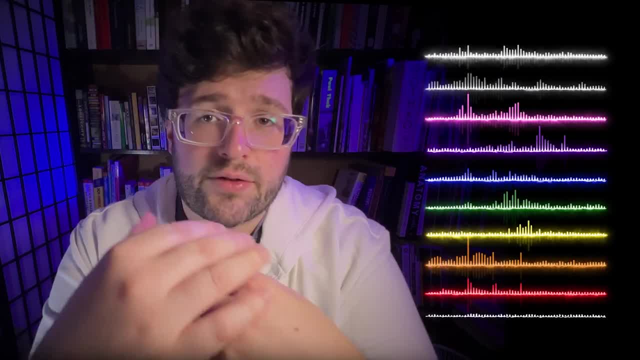 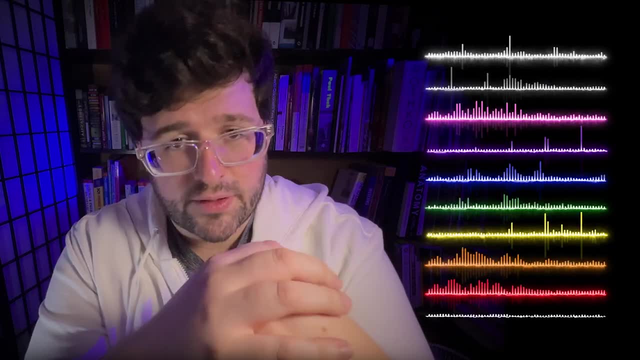 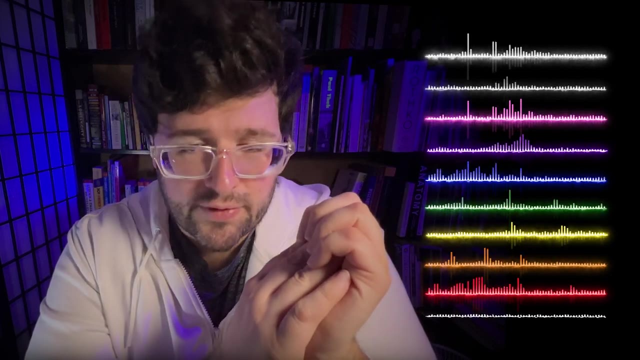 white noise actually has a variety of different categories that vary in loudness, frequency, spectrum and intensity. In the audio engineering and telecommunications world, there are more specific terms that describe various noise signals. These labels are part of the noise spectrum and can also be considered the color of noise. Different colors of noise have significantly different 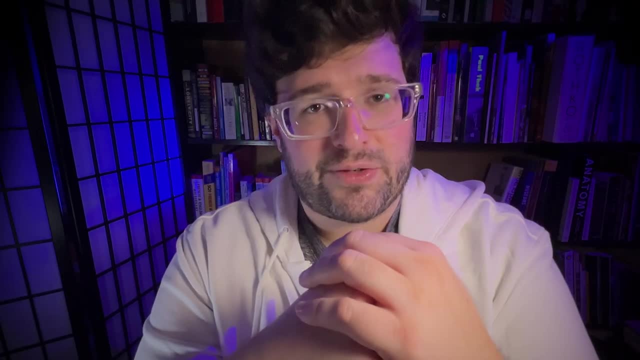 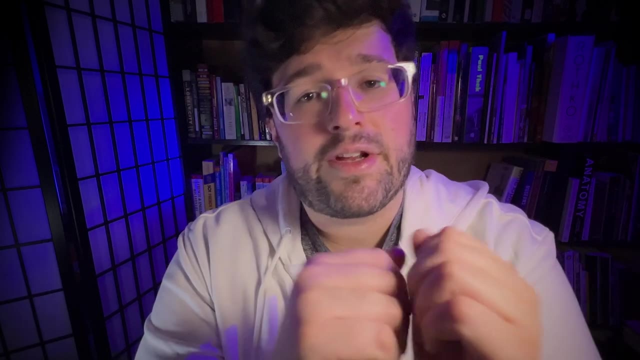 properties. Now, to keep things simple, we won't go over the technical ranges for most of these different sounds, but we'll run through different colors and discuss some of their differences. My personal favorite is red, also known as deep Brownian noise, But you might like pink noise or 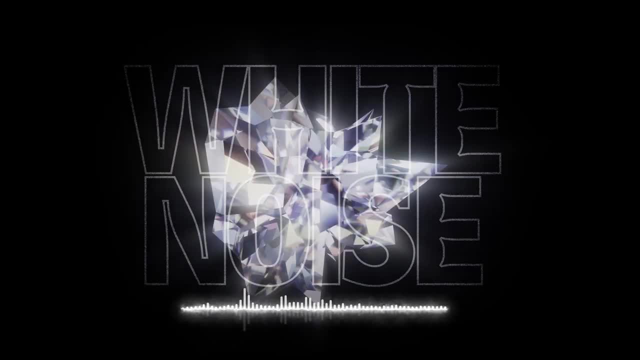 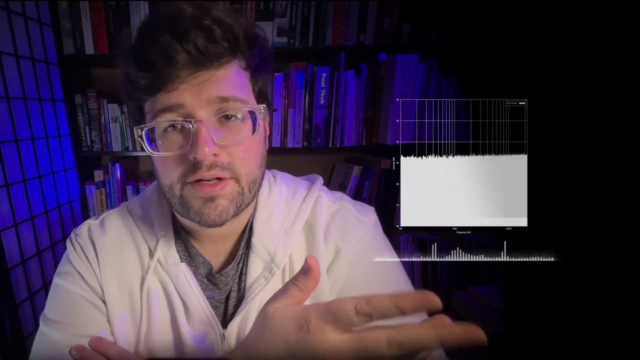 even yellow noise. So let's check them out. White noise is a random signal consisting of equal amounts of all frequencies in the human hearing range, That's around 20 hertz to 20 kilohertz. It's often described as sounding like static hissing, or white surf is used for sound. 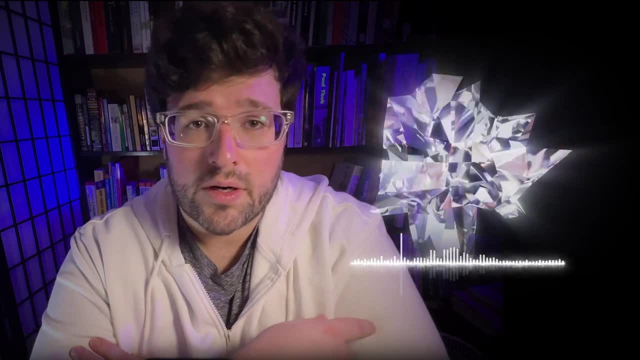 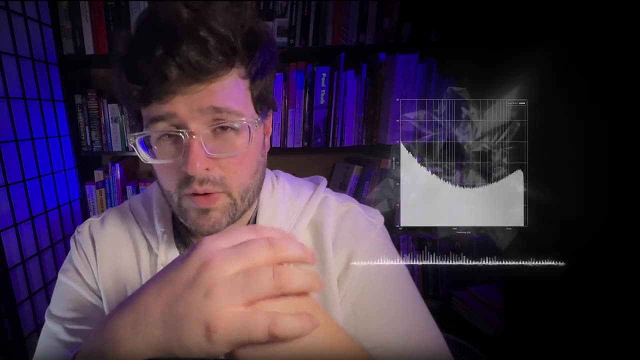 masking, And again, it's not always the same. It's often described as sounding like static hissing or can help some people fall asleep or concentrate better. Gray noise is like white noise, but it's altered to attempt to follow an equal loudness contour. The result is that gray noise contains 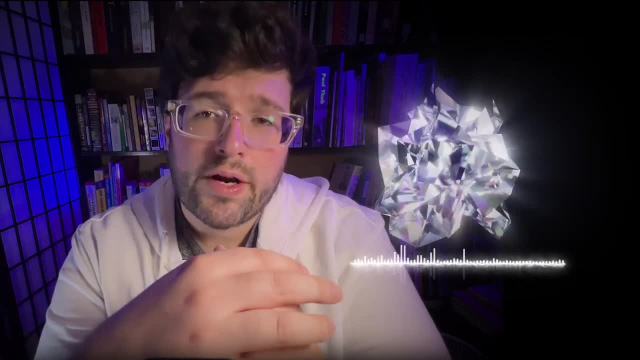 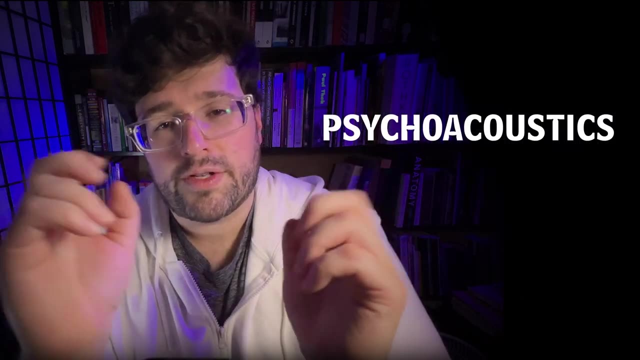 all frequencies with equal loudness, as opposed to white noise, which contains all frequencies with equal energy. The difference between the two is the result of psychoacoustics, or, more specifically, gray noise tries to adjust white noise so that it sounds like all frequencies. 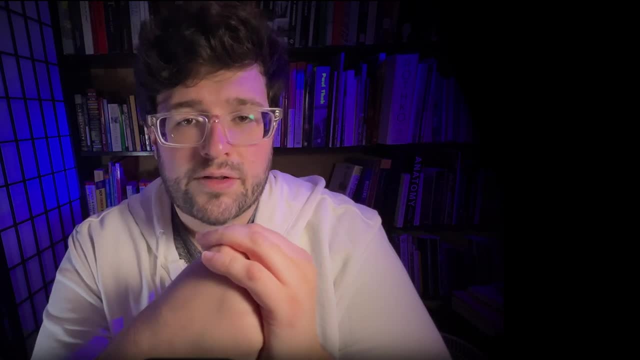 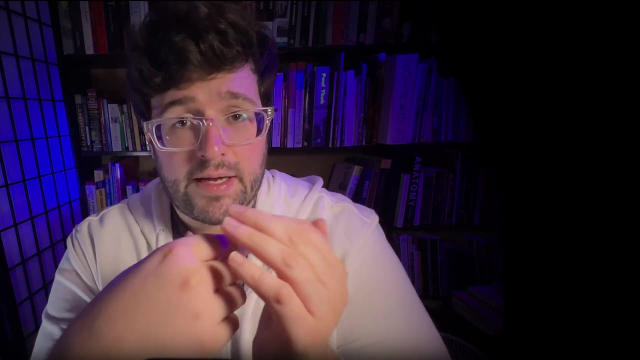 are the same to the human ear. This is because human hearing is more sensitive to some frequencies than others, Since loudness curves depend not only on the individual but also on the volume the noise is played at. there's actually no one true gray noise, But there is a simpler approximation. 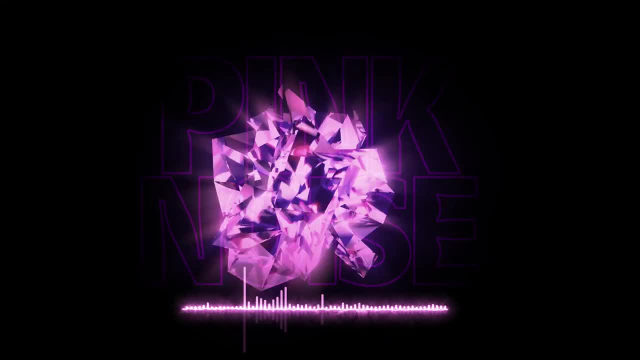 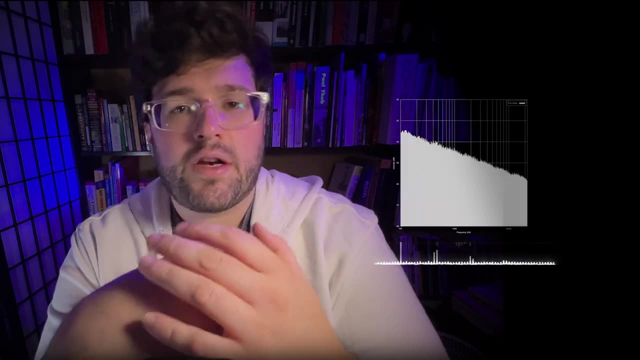 of an equal loudness noise, and that is pink noise. With pink noise each octave interval, halving or doubling in frequency, carries an equal amount of noise energy. It kind of sounds like a waterfall and is often used to tune loudspeaker systems and professional audio. 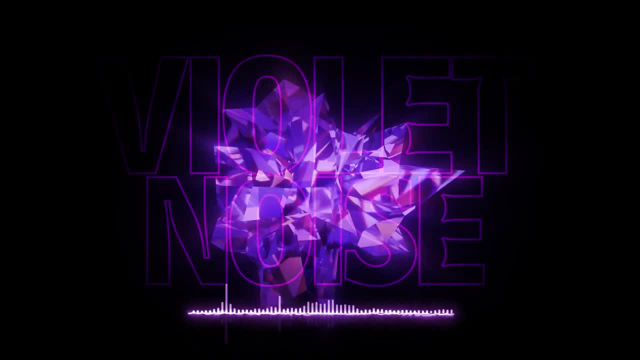 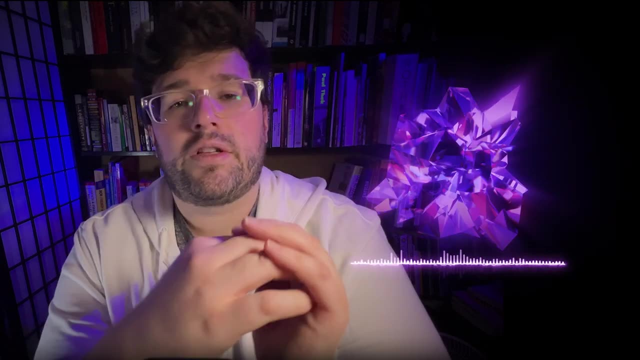 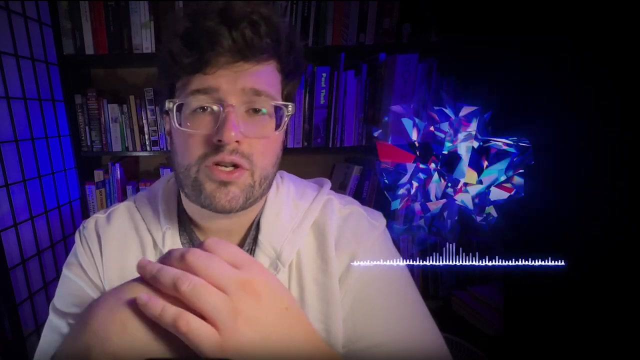 Since we're at pink, let's move to purple. Violet noise, also called purple noise, is similar to white noise, but it's shifted higher. This color range is primarily high frequency noise and sounds like a lighter and higher pitched hiss. Blue noise is also called azure noise. It's a scientific definition that involves